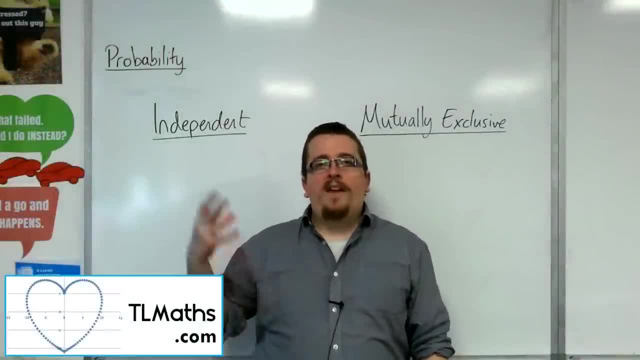 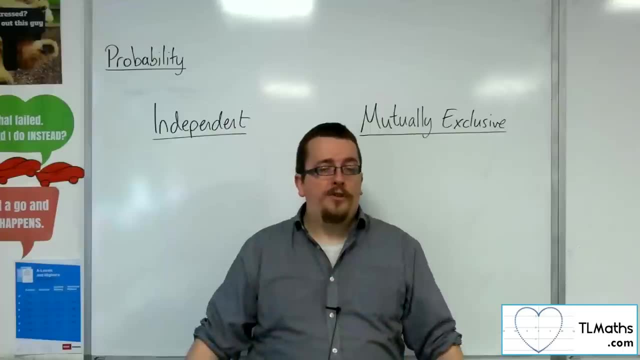 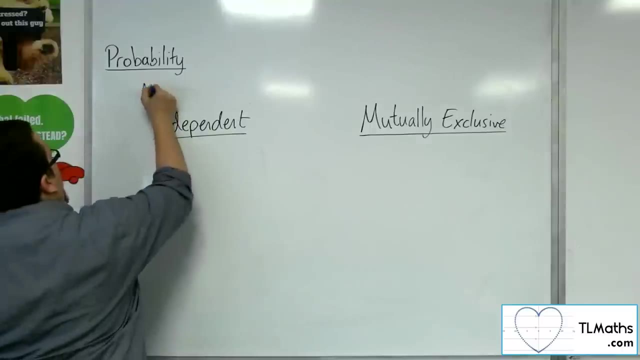 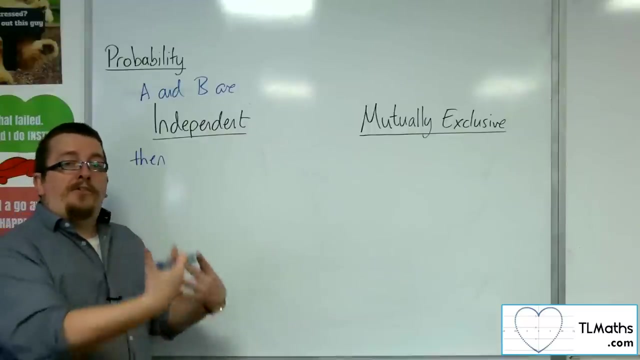 A common misconception in probability is that independent and mutually exclusive are synonymous, that they mean the same thing. They do not. OK, we must make that clear. So if two events, A and B, are independent of one another, then that means that if A were to happen, that doesn't mean that B is going to be any more likely or less likely to happen, and vice versa. 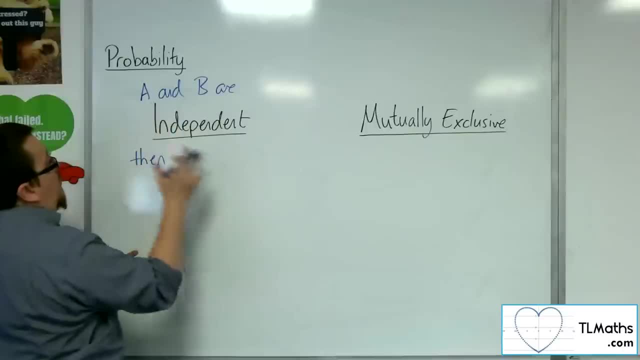 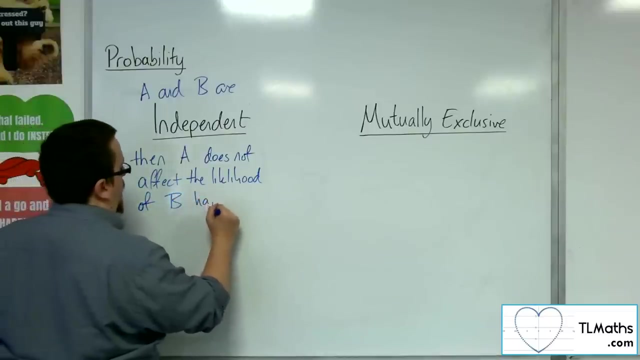 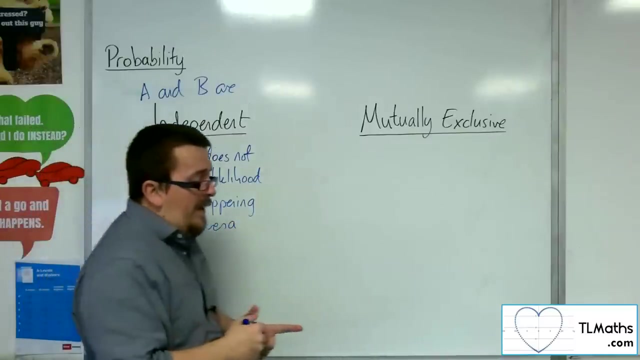 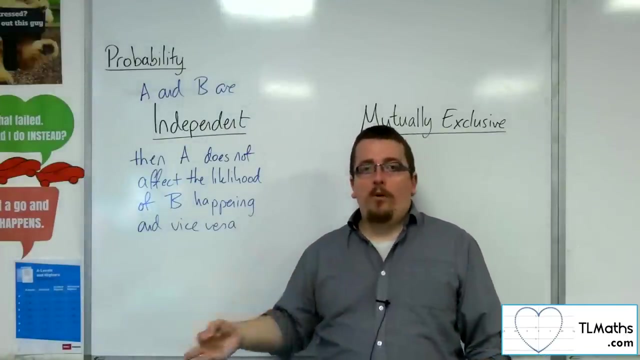 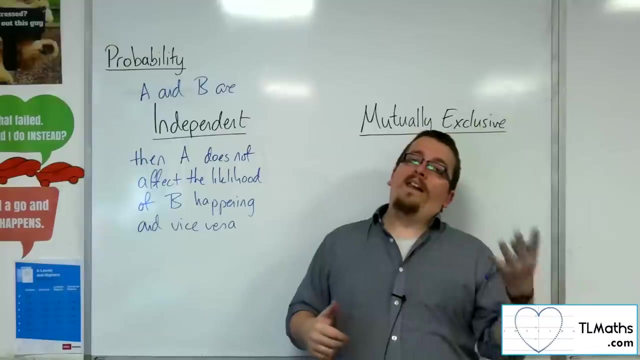 OK, so that would mean that A does not affect the likelihood of B happening, and vice versa. So let's say that there is a game that you're playing where you win if you roll a six on a fair, six-sided dice And you've got to pull an ace from a pack of 52 playing cards. 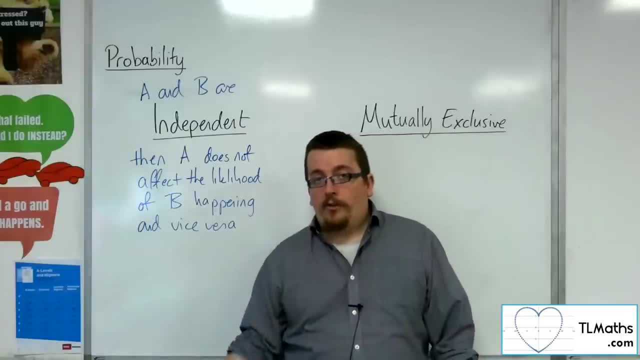 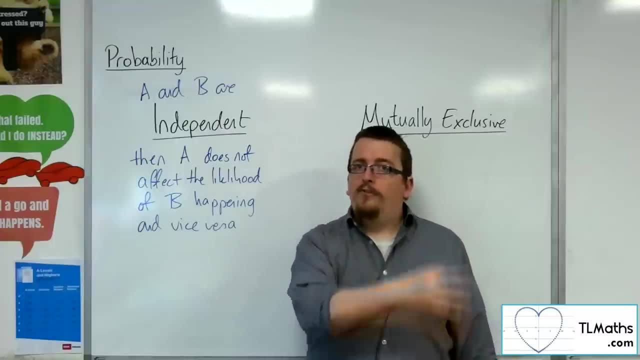 OK, if you roll a six on the dice, that does not then affect the likelihood of you pulling an ace from the 52 card pack. OK, the two events are completely independent of one another. One will not affect the outcome of the other. 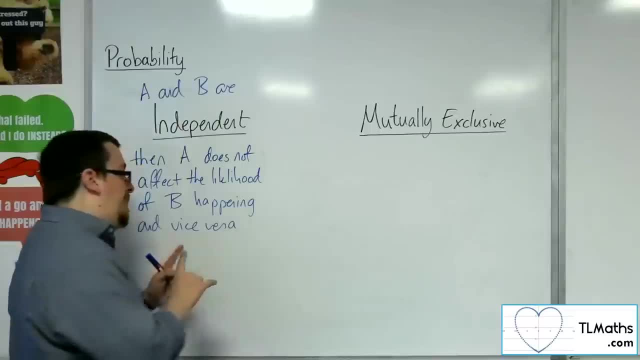 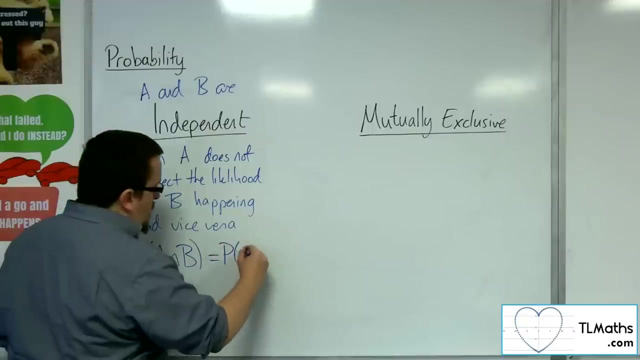 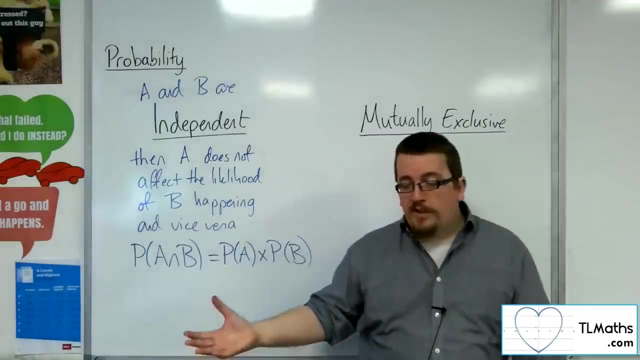 OK, OK, that's what we mean by independent events. And subsequently, if those two events are then independent, then what that means is that, in order for the intersection to happen, then that means that you can multiply the two probabilities together. OK, so in other words, if we go back to that game of rolling the six, so the probability of that is one sixth. 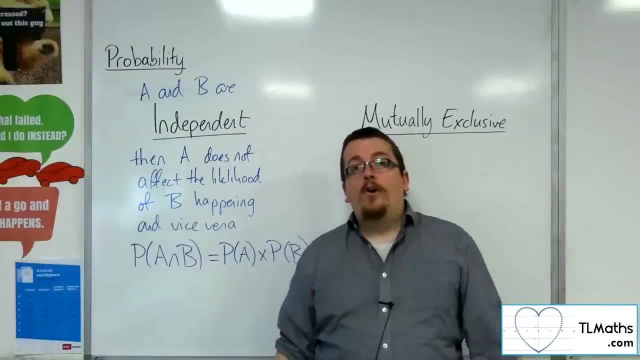 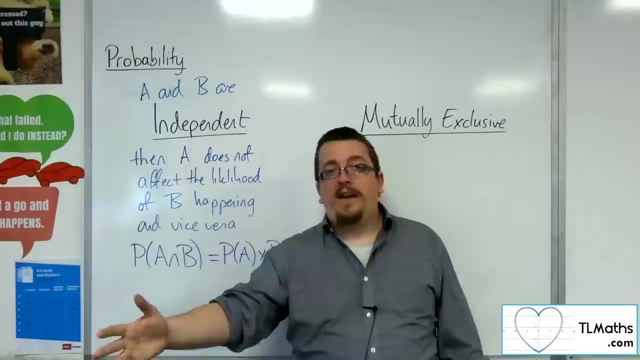 Of getting a six, And the probability of picking an ace from a pack of 52 playing cards is four out of 52, or one out of 13.. So you'd have one sixth times one thirteenth, And that would be the probability of winning the game.